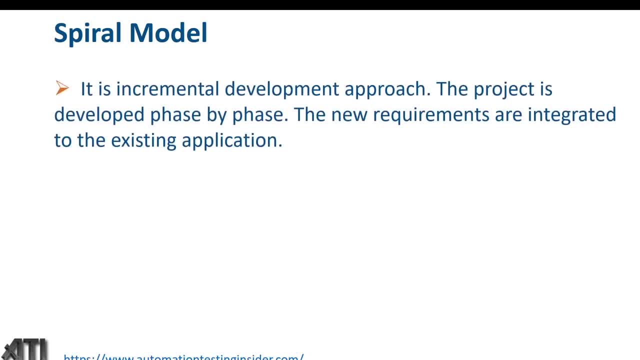 So let's get started. So it is incremental development approach. is incremental development approach? So you have seen, in iterative development approach, like we used to develop the product based on, based on the requirements, Like we prioritize the requirement and we develop module wise, module one, module two, like that. So that's why it is called incremental development approach. 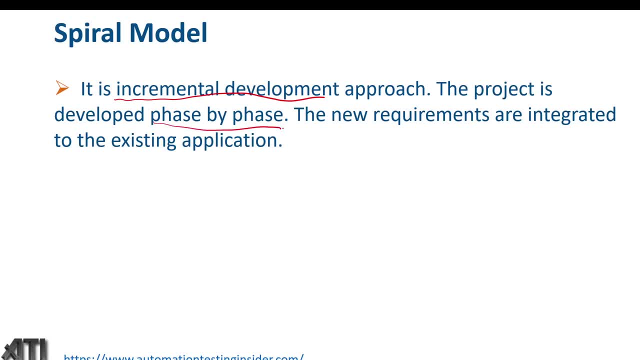 The project is developed phase by phase, is by phase, The new requirements are integrated to the existing application. So, as I have discussed, like module one we have certain requirements And then in module two we'll add some more requirements, and so on. 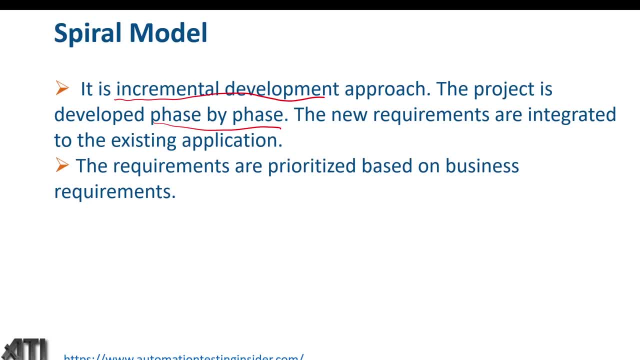 The requirements are prioritized based on business requirements. this is a risk-driven software development process model. so, as i have discussed like, this is the combination of waterfall model and iterative development model, but there is an extra factor like risk analysis, so it's risk. there is a high percentage of risk analysis in. 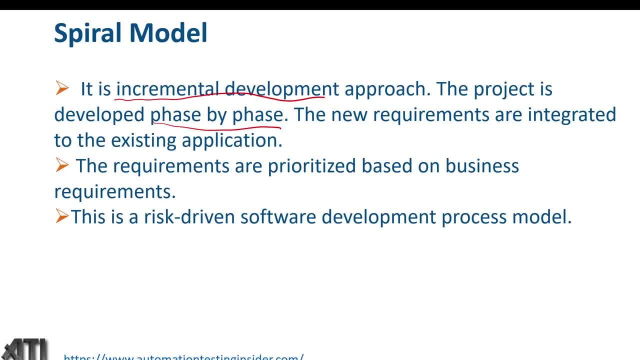 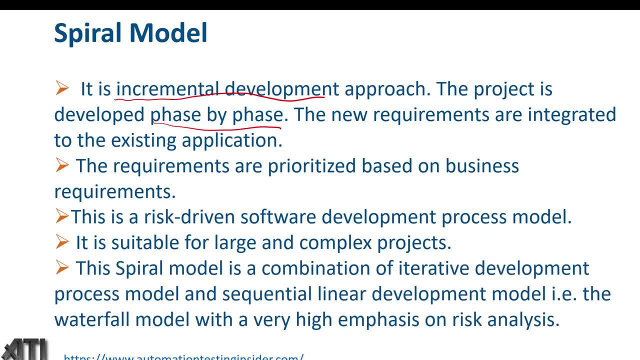 spiral model, so it is also called like risk-driven software development process model, so it is suitable for large and complex projects. this is spiral model is the combination of iterative development, iterative development process model and sequential linear development model. that is, waterfall model with a very high risk, high emphasize or risk analysis. 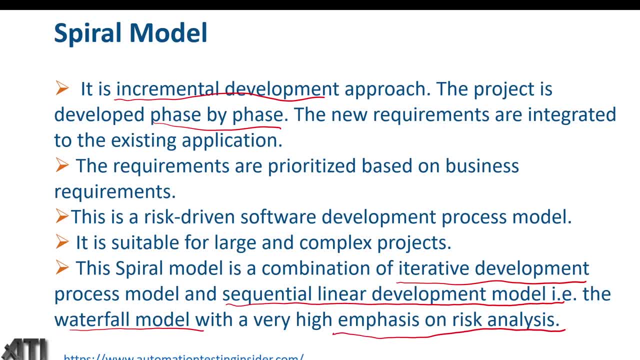 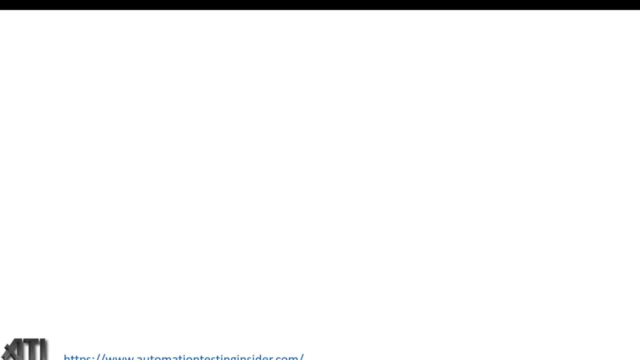 so this is, uh, there, these are the some notes about spiral model. now let's talk about in detail, like what is a spiral model with the help of diagram. so there are four phases in a spiral model. so first phase is planning. we have first phases planning and then we have risk analysis. 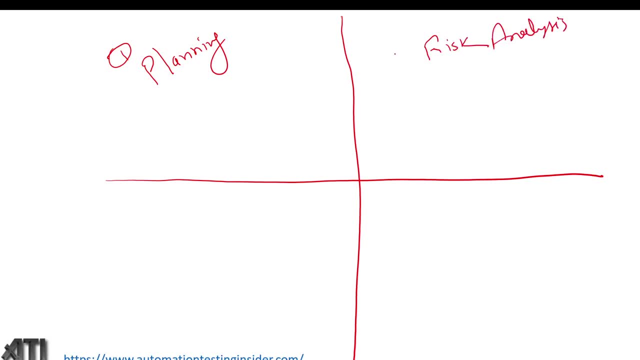 third would be coding and testing, or you can call it as engineering as well. engineering, or you may call it as implementation. this could be etüm eng to 뭐 or implementation. so the third phase you can call it as coding and testing or engineering or implementation. and the fourth one would be evolution. 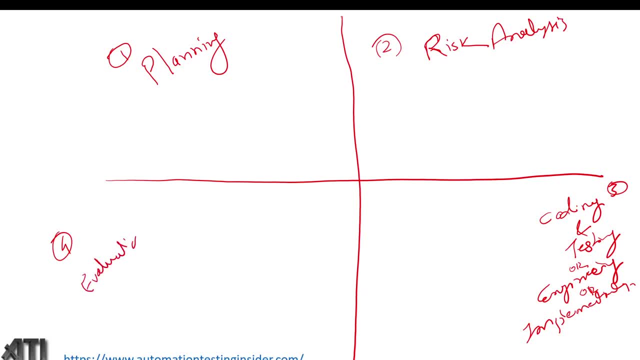 evaluation. so evaluation is done by, uh, by customers. they'll profile you and then suddenly the author says: good veiuki, hey boys, and 그럼 provide the feedback. so let's start with the planning phase. so yeah, it starts from here. so suppose we have we got some requirements from client and, in this particular phase, planning. 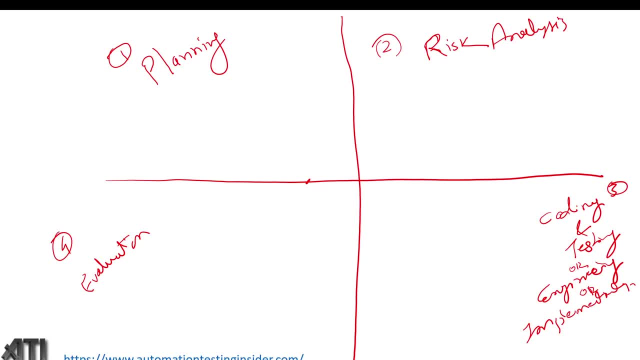 phase. what happens is ba works with customer to get the requirement and with the help of project manager, they, uh, they used to estimate the project and do the complete, uh, the planning of the project. so let's say we have divided our requirements into different modules. so right now we are 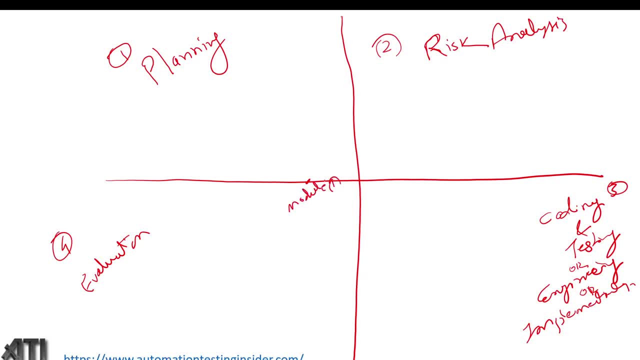 working on module one. this is module one, so this phase will start like this: now we need to do risk analysis for the module one, so we'll do risk analysis over here. so first of all we need to understand like what is risk? so risk is the positive possibility of something bad happening and you can say like it involves 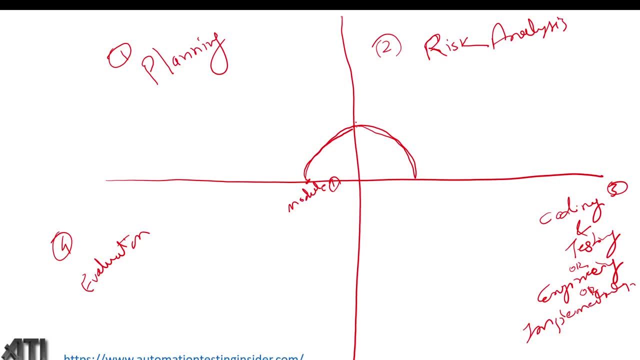 uncertainty, uh events like it may or may not happen in the future. so there are certain phases in risk, like certain steps to resolve the risk, like we have identification of the risk, evaluation, prioritization of the risk, and there could be different project related risk like scope related. 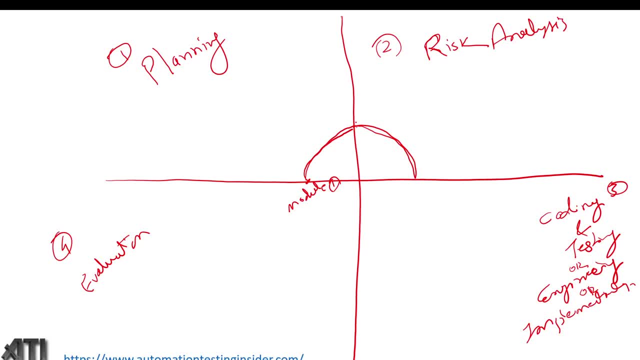 risk and cost related. we have schedule related as well and lack of clarity in the requirements, uh, resources unavailability. so these are the different risks. uh, we have first related means. if cost, it is the at higher side, so that will be a risk. we will do all kind of risk analysis. 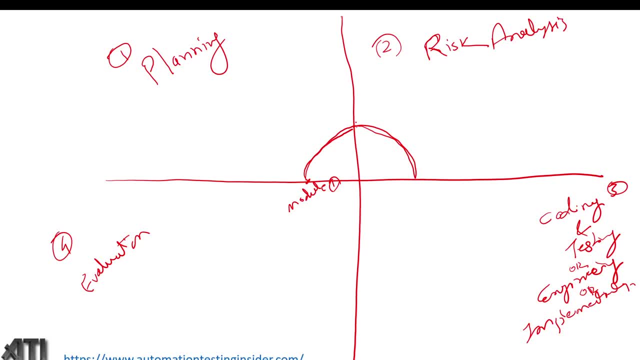 in this particular phase. so do not worry about guys like risk, because risk analysis is a separate uh topic we can discuss later on. so for now you can understand like these are the different risks, like whatever i have talked about related to project. so we'll do all kind of analysis over here. 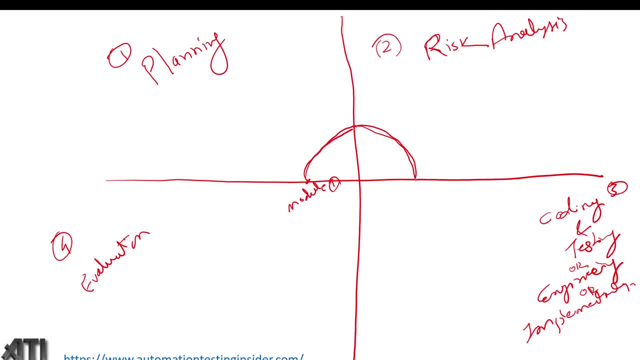 so risk analysis for module one is done now coding and coding and testing will be done in over here. so whatever requirements we got will do the coding developer will do the coding and they will implement the coding and then they'll send it to testing team for testing that particular module. 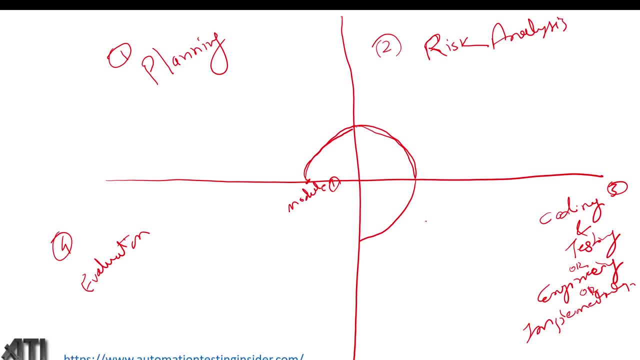 so we'll do the testing of module one over here. after successful- once successfully uh tested module one, then we'll go for the release and we'll do the release over here. so model one will be released over here and based on custom, our reviews and feedback. reviews and feedback. 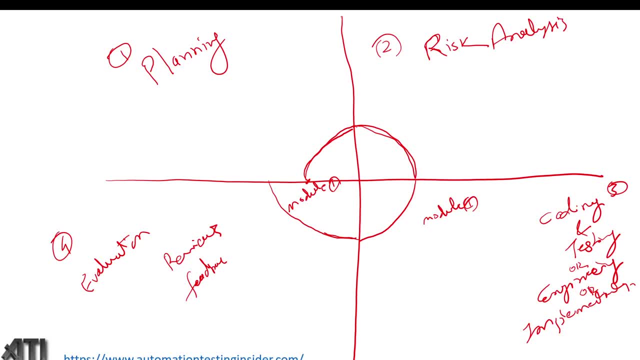 we'll work upon module 2, so we'll we may add some more requirements. uh, we can change the requirements from module 1, we can update the requirements of module 1 and we'll work with the new requirements from module 2 and then we'll start module 2 over here and then same process. 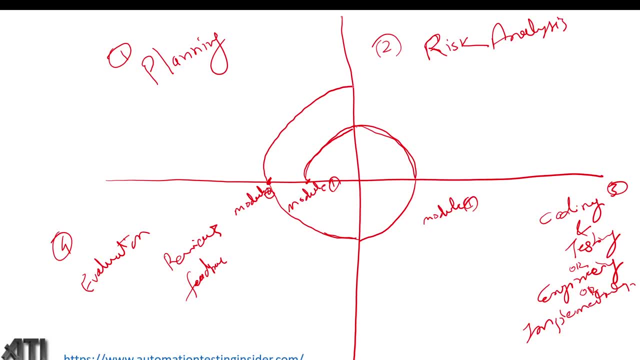 will go like this planning phase again will do uh, the planning for module 2 and the same thing like risk analysis for module 2 will be done over here and then coding of module 2 and developer will integrate module 2 with module 1 and we'll do integration testing of module 1 plus module 2 over here. 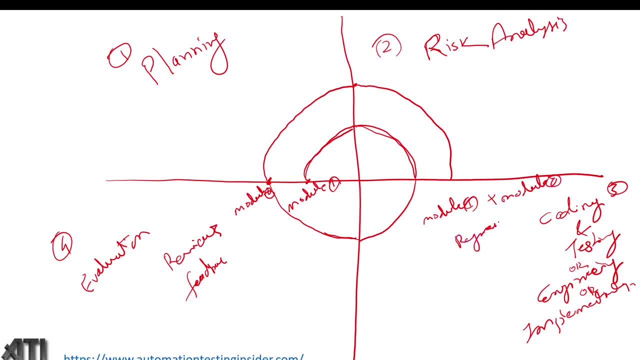 and we'll do regression for module 1. so we'll make sure that the changes, like changes of module 2, does not affect the module 1. so that's the reason we do the integration uh in regression testing over here. don't worry about different testing like integration or regression testing. we'll discuss. 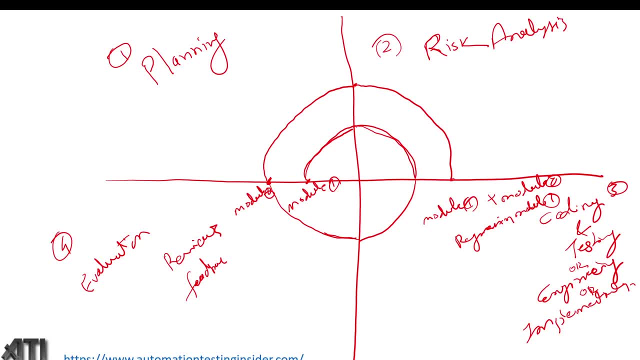 in coming videos, once testing and everything is done for module 2, and then we'll deploy module 1 and 2 over here. module 2, 1 and 2 integrated and we deployed successfully and we will work for module 3 over here. so this is how we'll keep working on module wise. 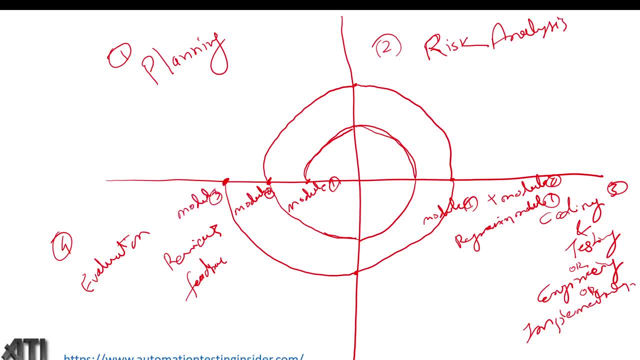 so let's say this is module, module 3. now again the same process will start: planning of the module 3, and then we'll do the risk analysis for module 3, module 3, and then again we'll integrate. we'll do the, the developer will integrate module. 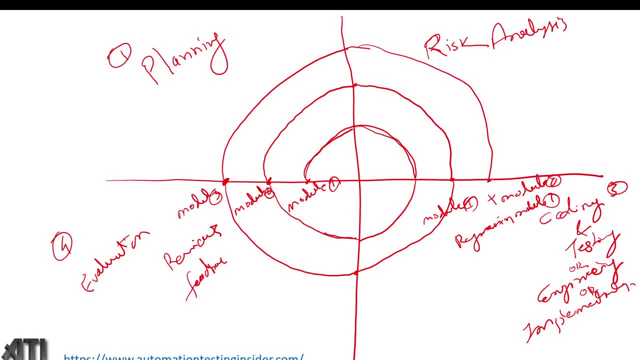 1, 1 and 2 with module 3, and we'll do the integration testing between among module 1, 2 and 3 and then we'll do the regression testing. like module 1 and module 2 does not get impacted, so on this process will go. so this is a spiral model, guys. so this is the combination of like. 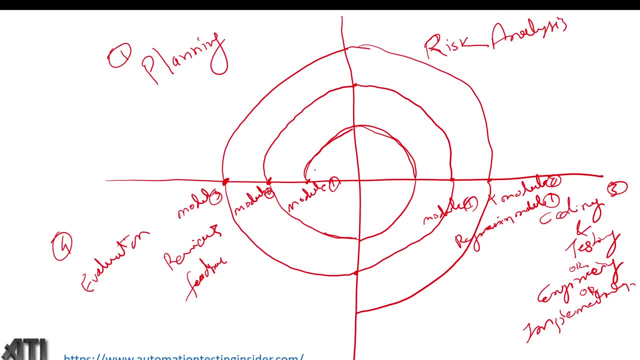 iteration, like iteration is there. you can see here, like we have: uh, addition is nothing but repeatable things. so we are keep repeating the same phases like planning, risk analysis, coding and testing and evaluation. we have four phases over here, so we will keep repeating, keep repeating all these phases. 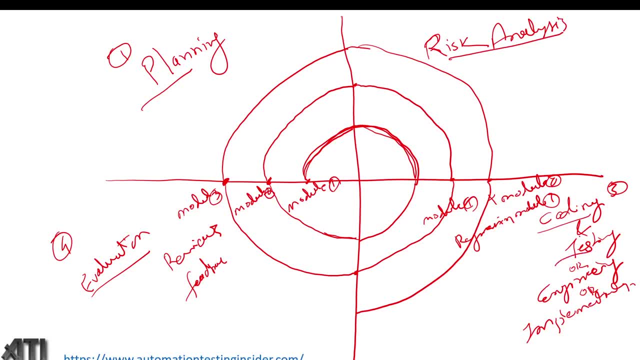 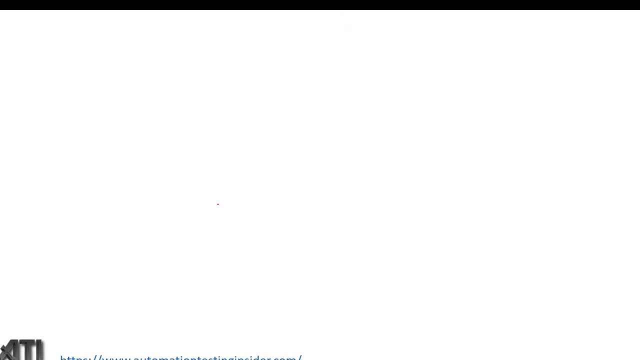 so that is iteration in a spiral model, and incremental is nothing. but we, we are adding module 1 with module 2 and module 3, so this is how we are developing the software. so this is about, uh, about spiral model. now, next, next we'll discuss, like, when to use a spiral model. 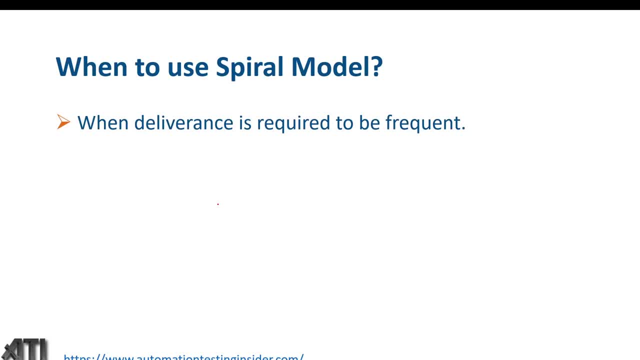 so when requirement is is when deliverance is required to be frequent, so we'll get when, when we get the frequent requirements from the customer. so we should go for parallel model. when project is large, of course, and when requirements are unclear and complex, so we can go for the spiral model, because in this